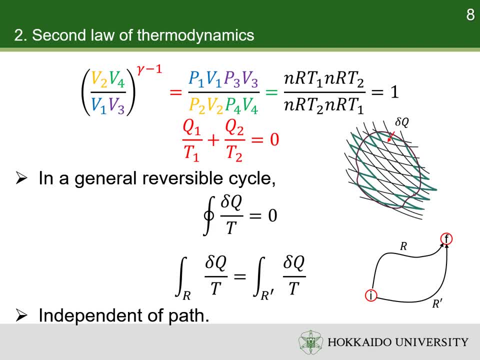 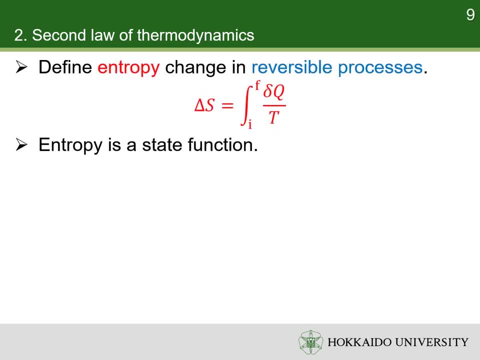 on the initial and final states. It is independent of the path. It is the change of a state function. We define this state function: entropy. The infinitesimal change of entropy, is delta Q over T. Accordingly, delta Q equals T? dS. Thus the first law of thermodynamics can be expressed: 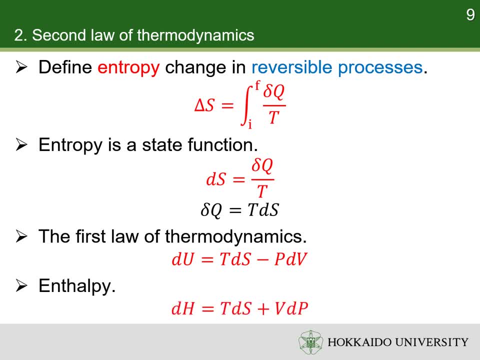 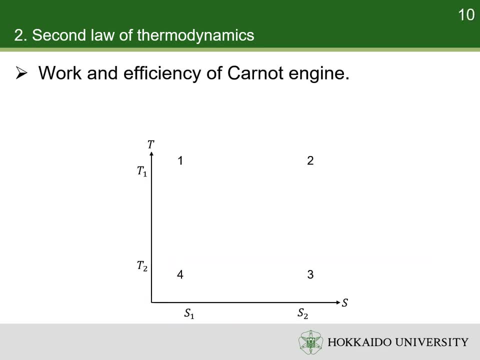 in the following form. Similarly, the infinitesimal change of enthalpy can be expressed in the following form. Now the Carnot cycle can be visualized with an entropy versus temperature plot. The isothermal processes are the horizontal lines, The adiabatic processes are the vertical. 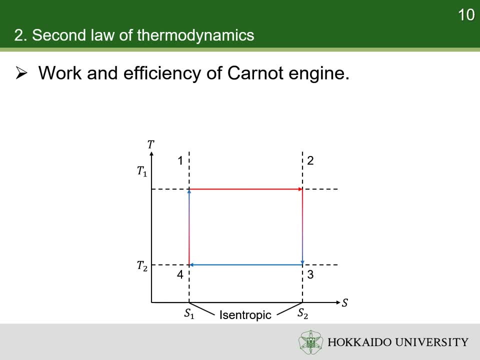 lines. Such both adiabatic and reversible processes are the horizontal lines. The adiabatic processes are also called isentropic processes. Some work is done by the so-called Carnot engine to the surroundings in a cycle, Since the internal energy change is zero. the opposite of work is 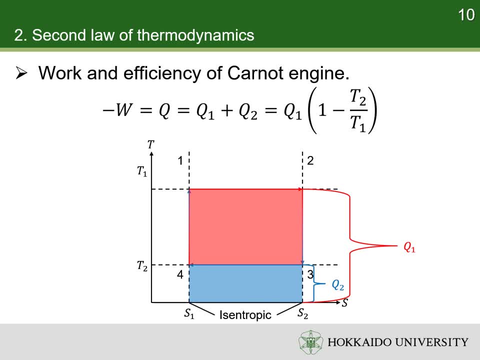 heat. In an isothermal process the heat is T times delta S. It is the area below the function. So Q1 plus Q2 is the difference in the areas of the rectangles. Pay attention to the sign of the heat. It depends on the direction of the process. It depends on the direction of the process. 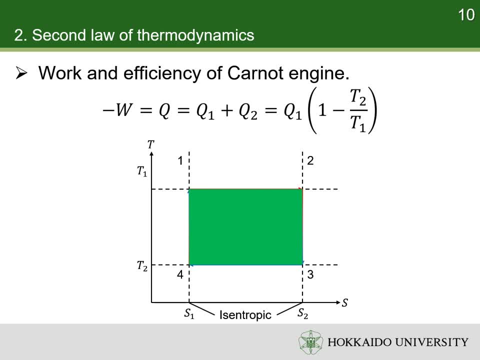 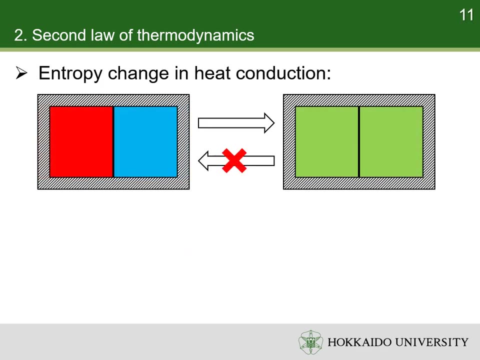 The work is the area inside the Carnot cycle. The efficiency of a heat engine is defined to be the ratio between the work done to the surroundings and the heat received by the engine. The efficiency of Carnot engine has such expression. Let's check the entropy change in heat. 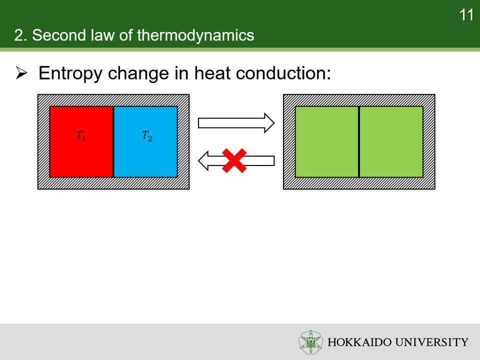 conduction Suppose, the temperatures of the warmer and colder water are T1 and T2, respectively. The heat passes from hot water to cold water. It is indeed a Clausius statement of second law of thermodynamics. It states that heat can never. 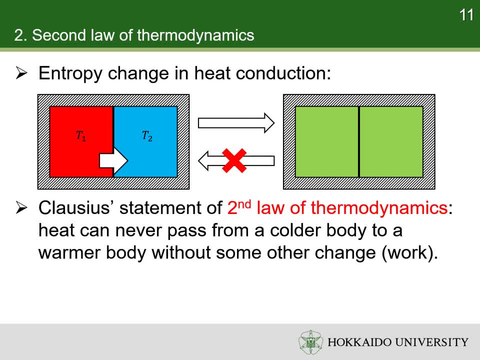 pass from a colder body to a warmer body without some other change. Here the other change is work. Suppose the heat of the warmer water is minus delta Q, Then the heat of the colder water is delta Q, We can find that the entropy change of the whole isolated system must be positive. 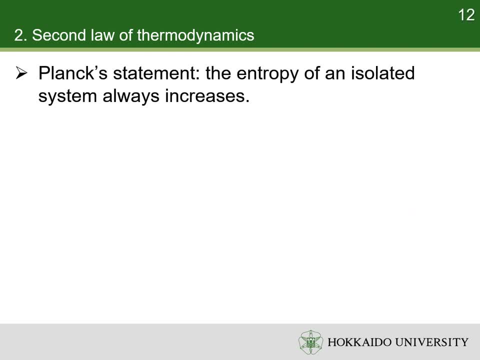 It leads to the Planck statement of second law of thermodynamics. It states that the entropy of an isolated system always increases. So entropy is called the arrow of time. In an isolated system, the direction of process depends on its entropy change. If a process increases the entropy of an isolated system, 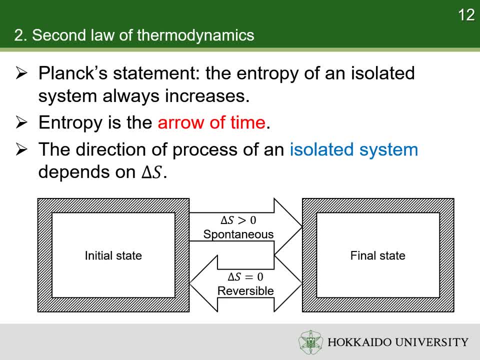 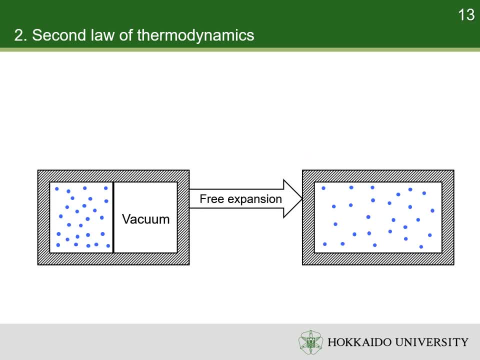 it happens spontaneously and irreversibly. If, in a process, the entropy of an isolated system is a constant, the process is reversible. Let's have a look at our previous example of free expansion. Since entropy is a state function, its change can be calculated using any pathway with the same 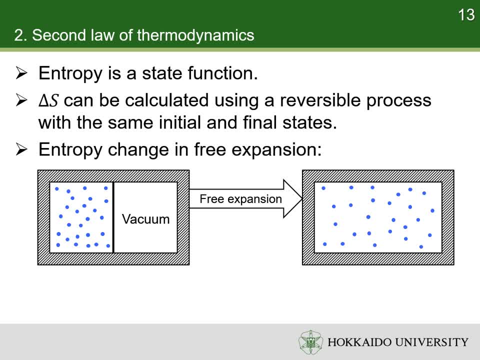 initial and final states, And because the temperature does not change during the free expansion, it is convenient to calculate the entropy change using an isothermal process. We can find that in a free expansion the final volume must be greater than the initial volume. 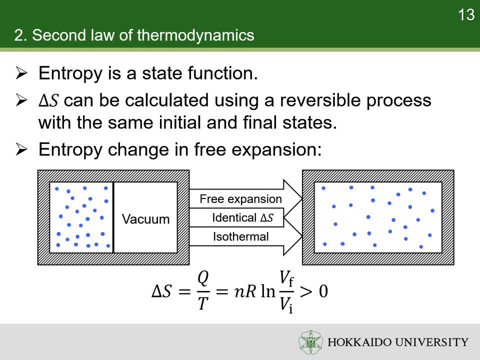 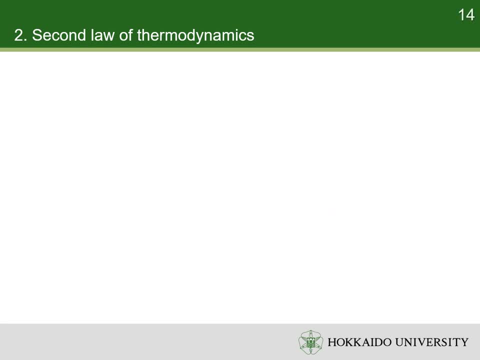 So the entropy increases in free expansion, That is in accordance with the Planck statement of second law of thermodynamics. There are various equivalent statements of second law of thermodynamics. Though I will not prove the equivalency between them Here, I show you two of them. Kelvin's statement of second law of thermodynamics states that 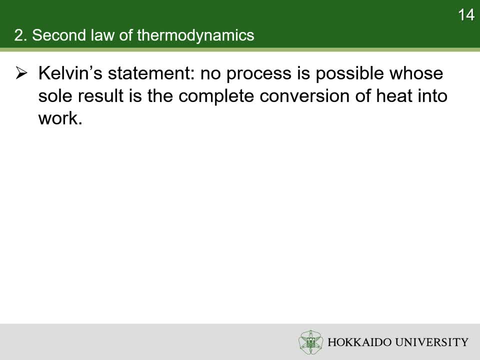 no process is possible whose sole result is the complete conversion of heat into work. The perpetual motion machine of the second kind, which spontaneously converts thermal energy into mechanical work, violates the second law of thermodynamics. So the entropy of an isolated system is irreversible. 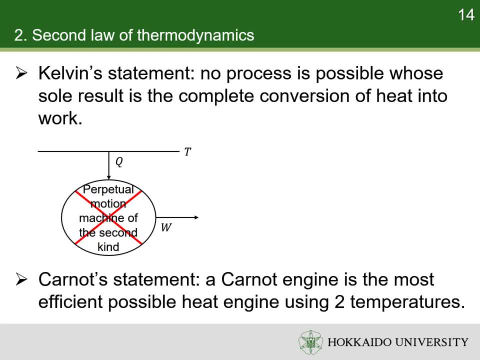 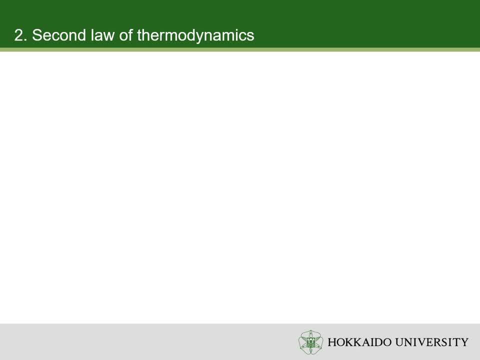 So it is impossible. The Carnot statement of second law of thermodynamics states that a Carnot engine is the most efficient possible heat engine using two temperatures. Here I have an example of a Stirling engine based on two isothermal and two isochoric processes. 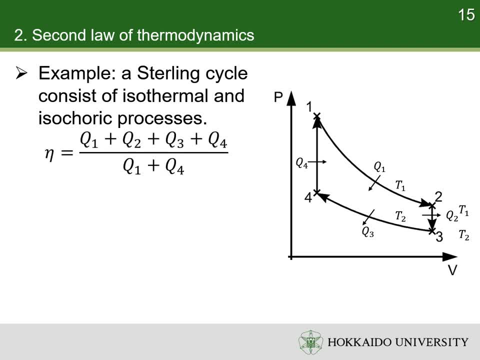 The efficiency is the ratio between the opposite of work and the heat received, where the opposite of work is the total heat. The heat of an isothermal process is calculated with the initial and final volumes. The heat of an isobaric process is calculated with the initial and final temperatures.